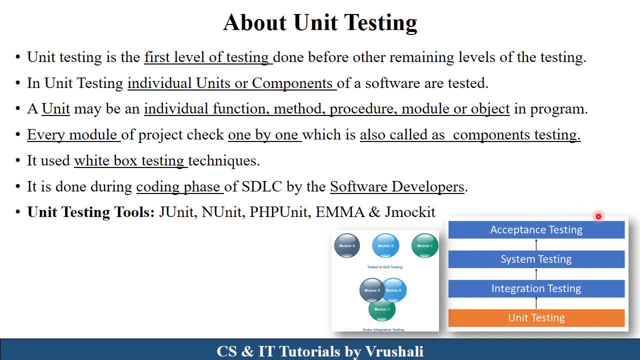 in testing process of particular project. See here in this image while developing a particular project. Unit testing is a first level. After that integration system and acceptance testing will be performed. Basically, unit testing perform on individual units or components of particular software. Now, what exactly units? See in your program. you have to mention different. 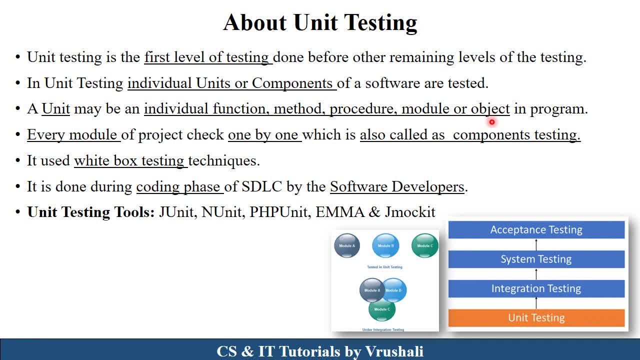 functions, methods, procedures, modules or objects- Right. So unit testing. perform on this all individual components, Basically every module of project, check one by one in unit testing. That's why, which is also called as component testing, This unit testing is used with white box testing techniques. 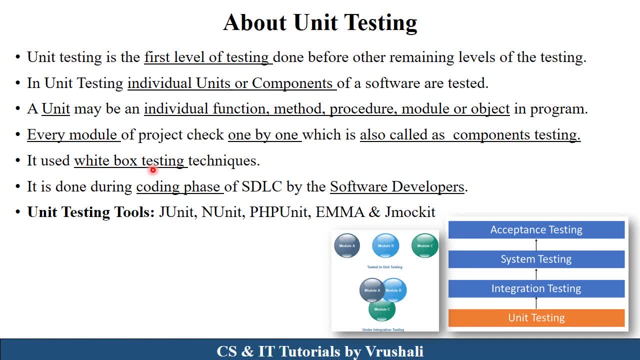 We already discussed white box testing in previous session. Basically, unit testing is work on internal structure, internal program and internal working of particular project. This unit testing perform in coding phase or implementation phase of software development. We have to mention here that unit testing is a first level of development. 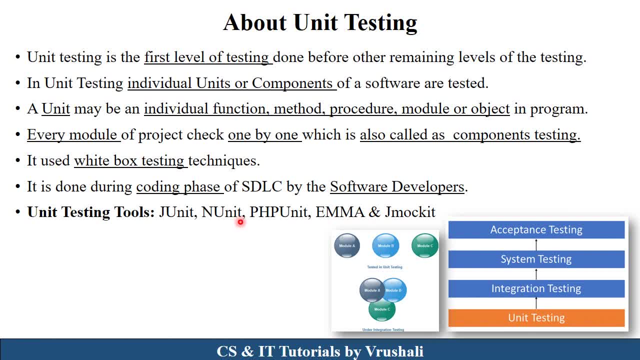 Now, here in this image, let's see all these different unit testing tools. Now this is all of the unit testing tools, like unit testing tool, which are available in market. There are different unit testing tools available in market, Like J unit, AN unit, PHP unit. 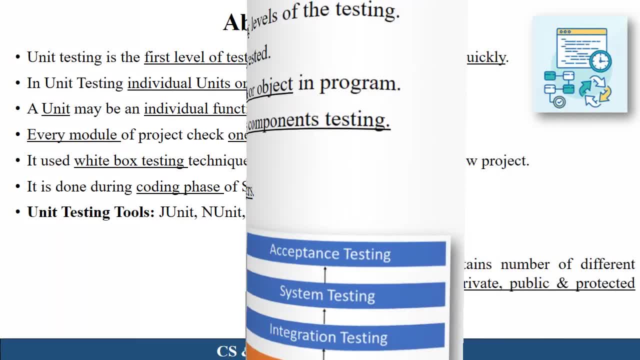 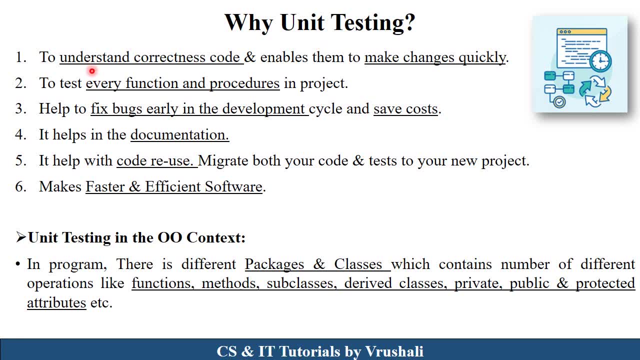 etc. These all tools are used by the tester to generate different types of test cases. Now the next point is why unit testing is necessary. See, due to unit testing, tester understand correctness and accuracy of your code. Now, here, in the first level of testing, you have to understand the types of test cases. 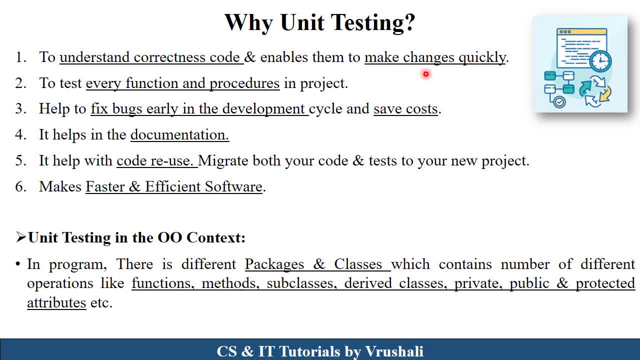 If there are any errors they easily make any changes quickly. Unit testing also test every functions and procedures mentioned in your program. Unit testing perform or find out errors at early stage of development. That's why they save cost and money. also See in particular project. suppose there are total three modules. 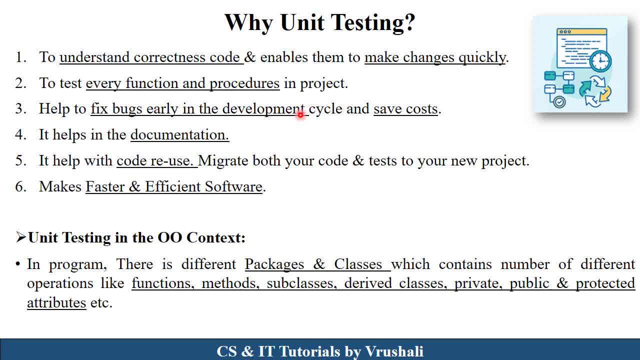 So developer work on module one side by side, they perform the testing. When they perform module two, also side by side, they perform testing on each and every functions, procedures and methods mentioned in particular program right. Then unit testing also help in documentation phase and also help with code reusability. 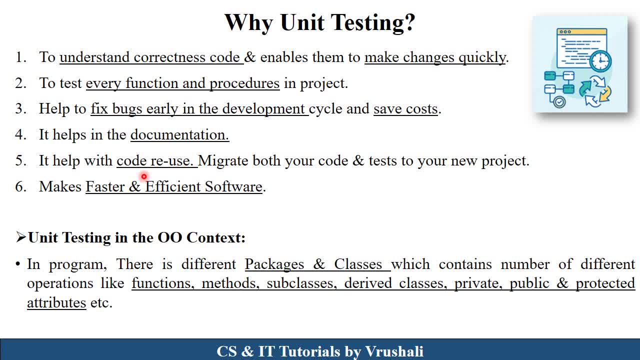 You can use same module, same code with another project. Basically it makes faster and efficient software. Now unit testing also understand some object oriented context. See, In your program you have to declare different packages, classes. under that classes there are subclasses, derived classes, right. 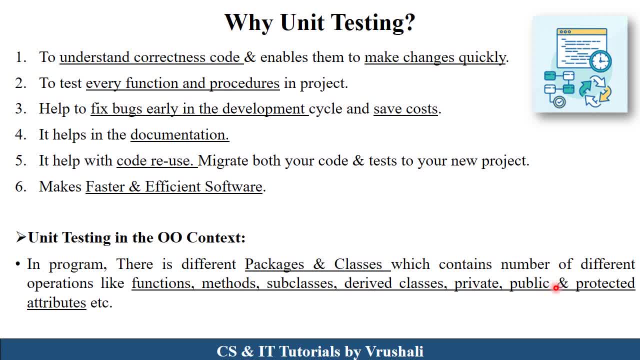 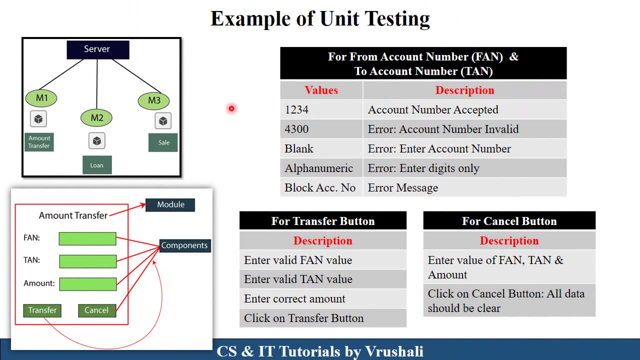 You have to declare different functions, methods, then private, public and protected attributes in your program. So unit testing, perform on this, each and every components, That every components will work properly or not. Now see here. this is an example of unit testing. 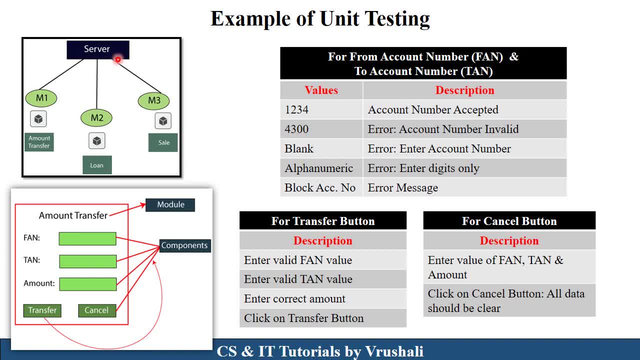 See, Suppose there is a banking service. Under that banking server there are total three modules. The first module is amount transfer, second module is loan related and third module is share related. So basically unit testing perform on each and every module and their functionality individually. 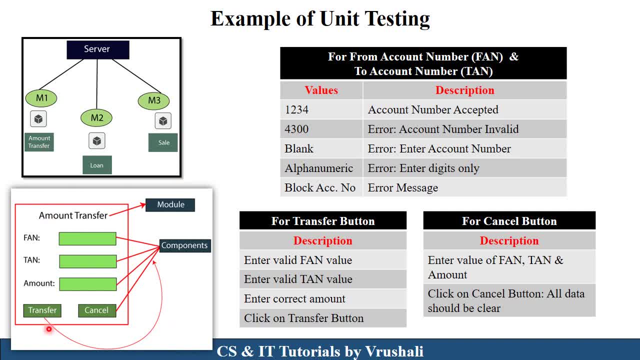 Suppose: the first module is amount transfer module. See here in this particular image: In amount transfer module there is a first from account number than to account number And mention amount here. After that there are two buttons, that is transfer and cancel, right. 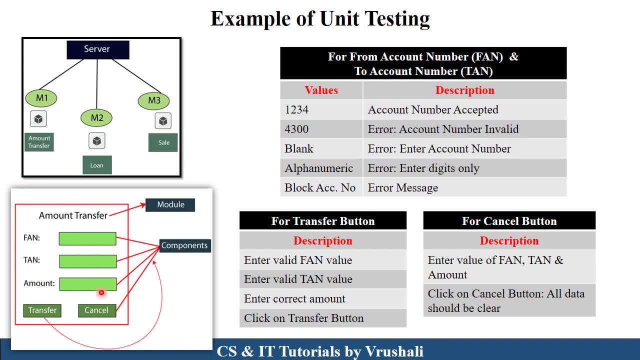 So this is a amount transfer module and there are various components or the features. Now tester generate different types of test cases on this features and functionality of that module in unit testing. How see here? Suppose there is a from account number and to account number? 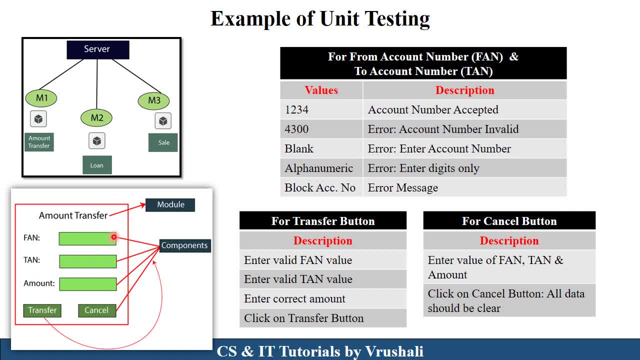 Okay. So for transferring money purpose, User need to enter money purpose. Okay, Valid account number only. Okay, Suppose they enter 1234.. So they will give the message account number accepted, Suppose they enter 4300 and this is invalid account number. 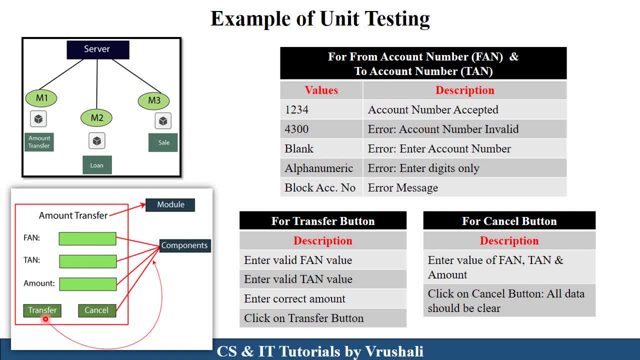 They will give you a particular error right. Suppose user click directly on that transfer button So at that time they will show the error. enter account number. Sometime user enter wrong account number or mention some alpha numeric value Like A, B, C, D in this way: 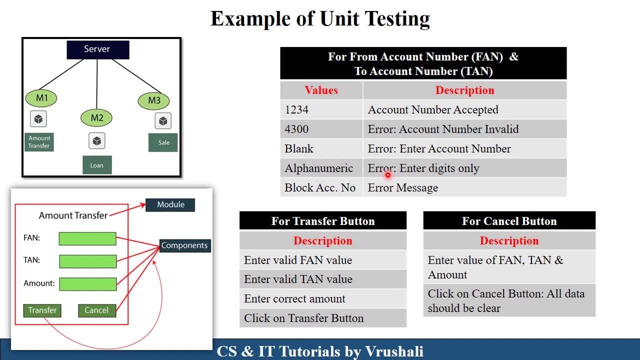 But account number always is in digits format, right? So at that time they will give you error: enter digits only. So this is called as test cases. They generate different types of test cases to test that a particular module is working properly or not. 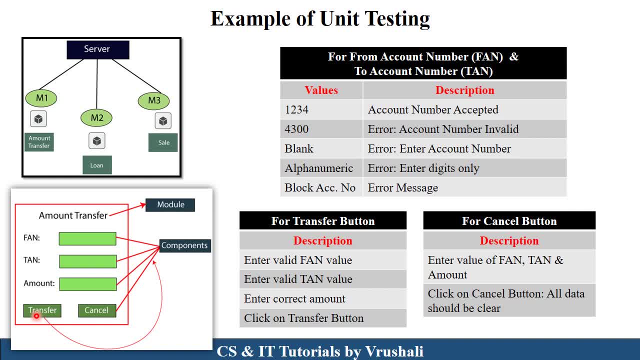 Similarly there is a transfer button. Suppose user enter valid from account number and to account number and correct amount, than only transfer button is work right. Otherwise they will give you error to enter account number or amount. The next thing is cancel button. when user click on cancel button, 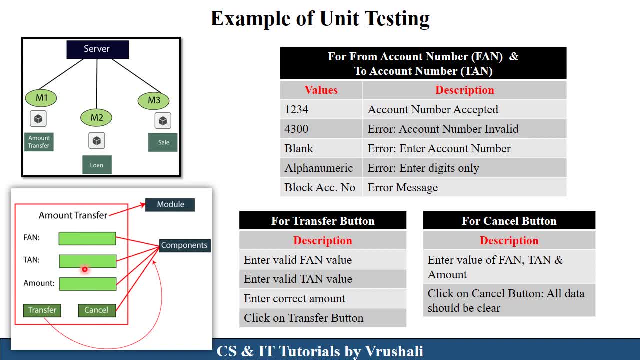 All data should be clear, right, So this is called as unit testing. Unit testing work on each and every module and their functionalities or components mentioned in your project. That's why they provide correctness or accuracy in output or the result. Now The next point is advantages of unit testing. 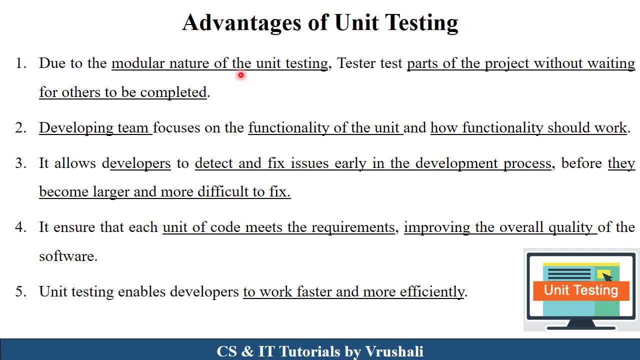 This unit testing, also called as modular testing because they work on module by module and their functionalities. Here developing team focus on each and every functionality mentioned on particular module and how this functionality should be work. Here developer find out all the errors or bugs at early stage of development, before. 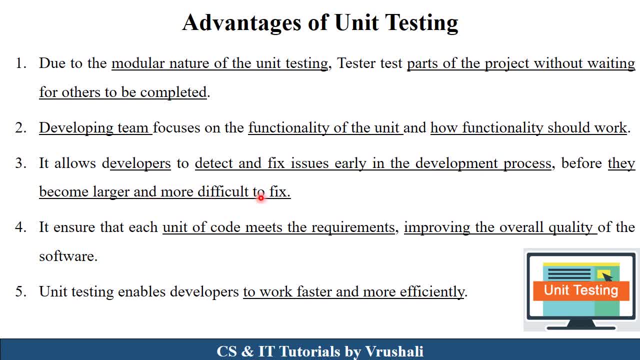 they become larger and more difficult to fix. This is the main advantages of unit testing. Unit testing also ensure that the output or the result it check as per the customer requirements or not. So unit testing basically improve overall quality of your code or the software. 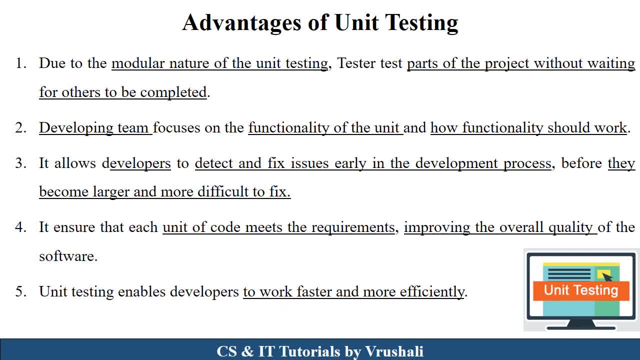 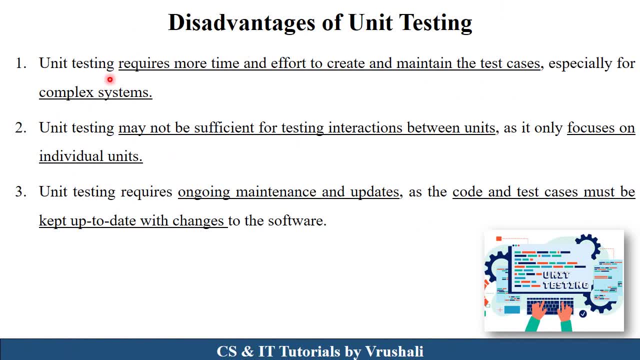 Unit testing also enable developers to work faster and more efficiently. Now the next thing is disadvantages of unit testing. See unit testing. work on each and every module and each and every module and their functionalities and each and every functionality mentioned on that. That's why it require more time and efforts to create and maintain different types of 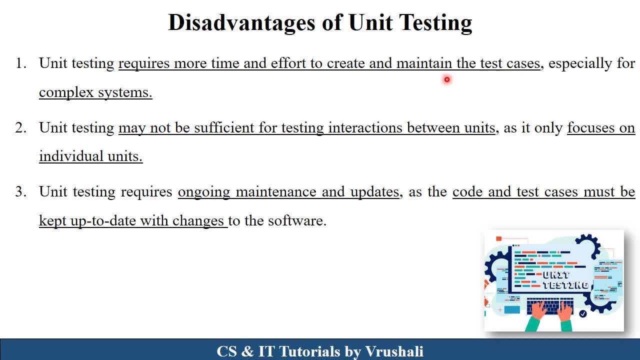 test cases. It is used for smaller system but it get difficult for the complex system. Unit testing also work on individual units, not a complete product or the complete program, And unit testing require ongoing maintenance and updates. See suppose customer requirements are changed At that time, code design, test cases also change right. 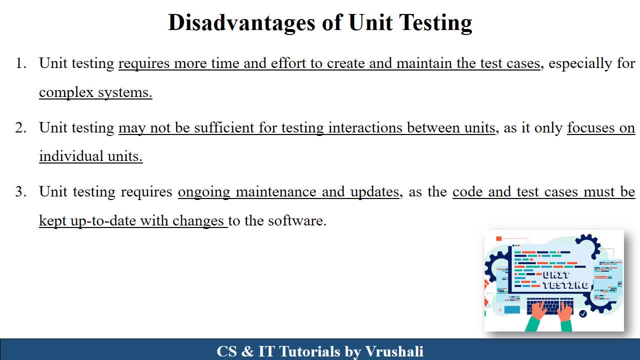 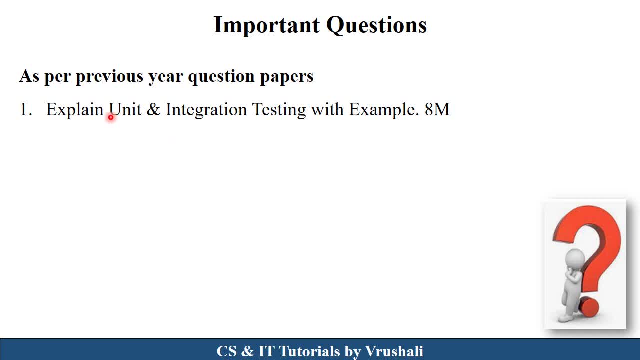 So that's why it require maintenance and updates every time. Now, as per your exam point of view in previous year question paper they have asked: explain unit and integration testing with example. So at that time you have to mention the some theoretical approach of unit and integration.